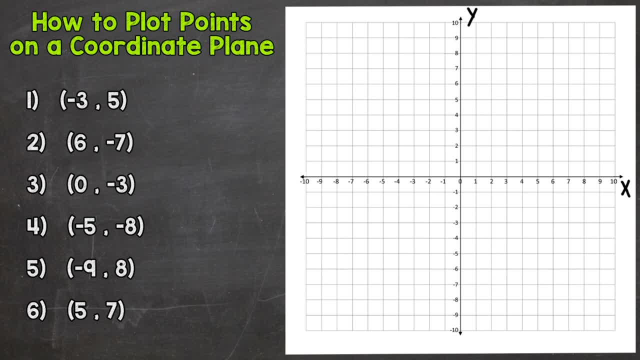 which one's the x-axis and which one's the y. we can get into plotting these points. So let's jump right in to number one. And we have negative three, five there, And the x-coordinate always comes first. So this negative three is our x-coordinate. 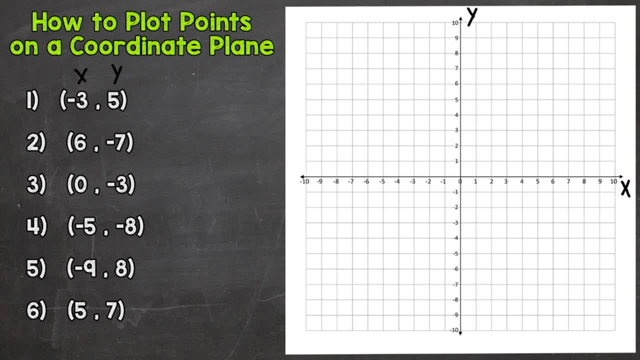 And the five is our y. Again, the x-coordinate always comes first and then the y. So now let's plot this point. So we always start from the center here, the zero, zero. And I'll put a circle around it: We always start from zero, zero, the center of our coordinate. 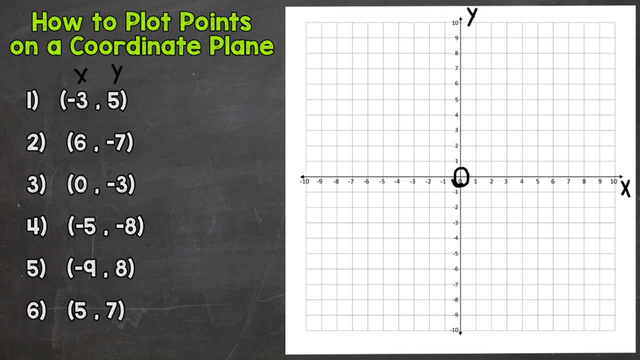 plane. And then we go over on our x-axis first And our first coordinate here is a negative three, That's our x. So we need to go left to zero, over to negative three here, And then we need to go up five because we have a positive five, So over negative three up. 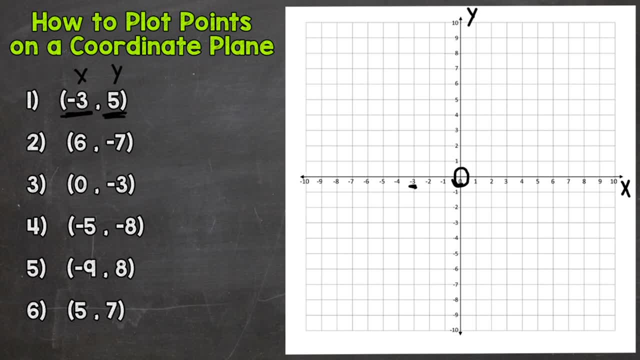 five, Always over, then up, And where the negative three and the negative three are intersecting, we plot our point And I'll label this negative three five. So let's go to number two. Our x is a positive six, And then we need to go down to negative. 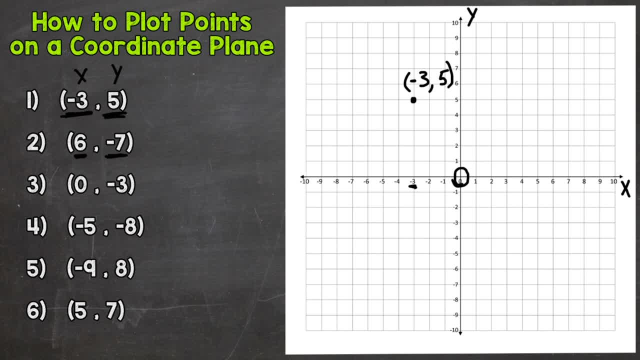 seven. So we start at our origin in the center And we go over six. So we find our positive six here And now we need to go down negative seven And we're going down because that's a negative seven, not a positive seven. So we go down, find where they intersect and plot our point. 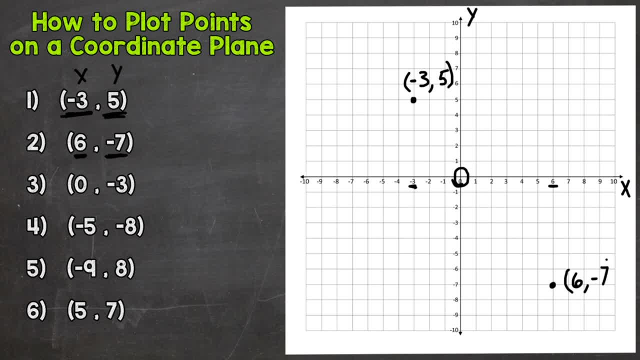 And I'll label our point six negative seven. So number three: we have zero negative three. So since our x-coordinate is a zero, we do not need to move And therefore the point is on our x-axis. So we stay right here at zero in the center. 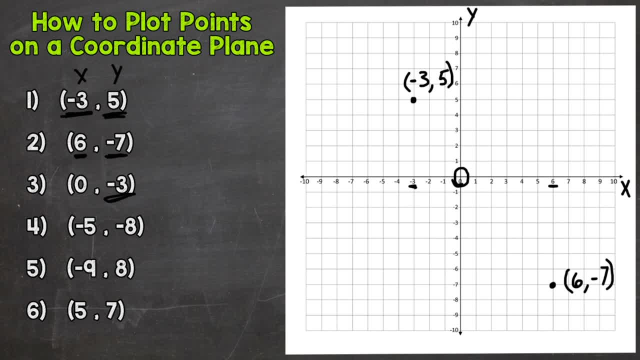 And our y is a negative three. So again, this is a negative. So we're going to go down on our y-axis to negative three And we plot our point And it's actually going to be directly on our y-axis, since we didn't move over at all. 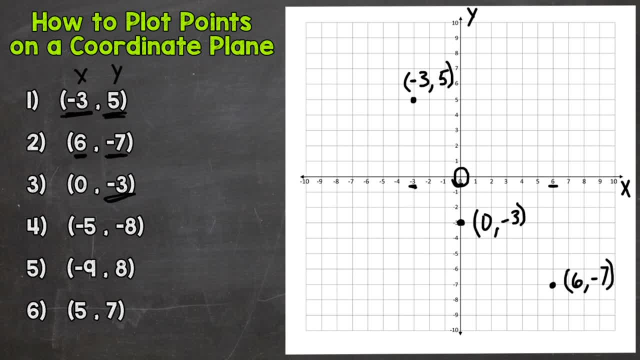 on our x-axis. So this is zero, negative three Aloha Number four. we have two negative numbers here: negative five, negative eight. So let's start in the center here and go over to negative five, And then we need to go down to negative eight and find where they intersect and plot our point. 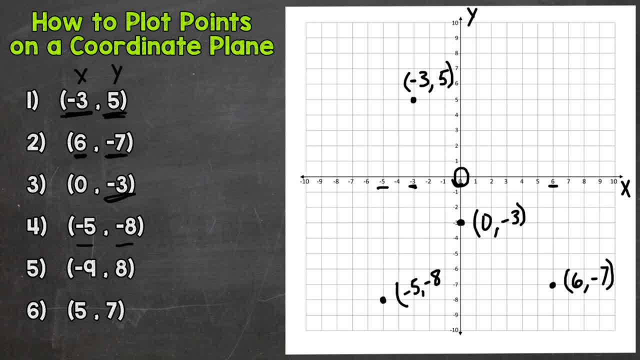 Then we'll label negative five, negative eight, Number five: we have a negative x-coordinate and a positive y-coordinate. So we start in the center, go over to negative nine and then up eight, because again that y-coordinate is positive. 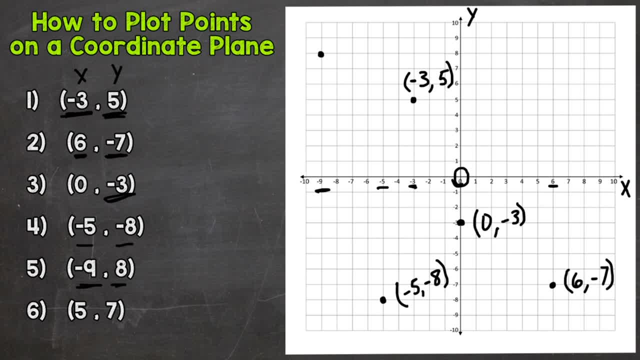 So we go up eight and plot our point. So negative, nine, eight. Lastly, we have two positive coordinates: five, seven. So we would go over to positive five here and then up to positive seven, plot our point and label five, seven. 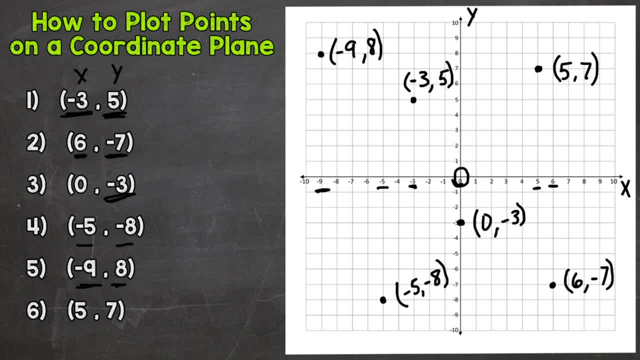 So there you have it. There's how you plot points on a coordinate plane. Just remember: x is horizontal, side to side, and y is up and down. So if you want to plot points on vertical, your x-coordinate always comes first, always goes side to side, then up or down. 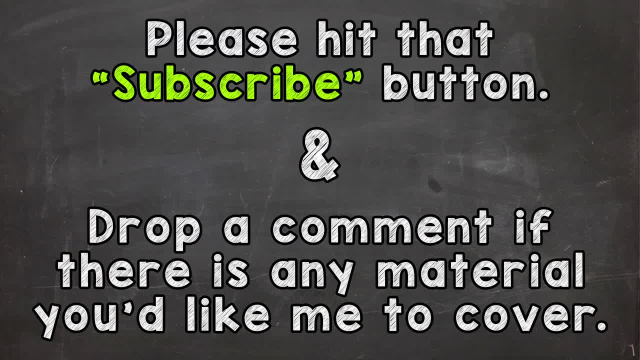 Thanks so much for watching. Until next time, peace.